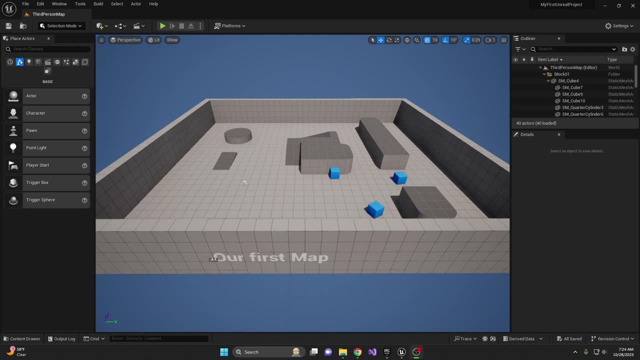 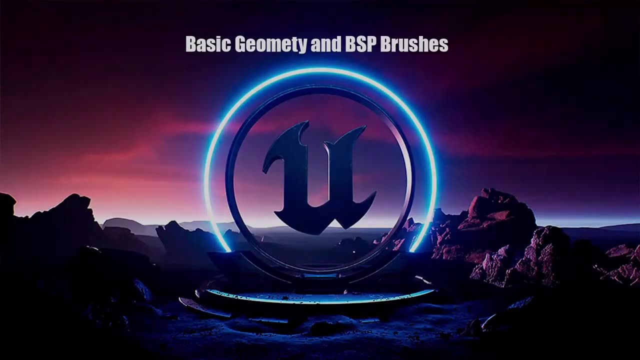 hit that subscribe button and ring the notification bell so you never miss out on unlocking the secrets of Unreal Engine 5.. Last time we took a deep dive into the viewport navigation. Now we're stepping it up with basic geometry and binary space partitioning brushes. 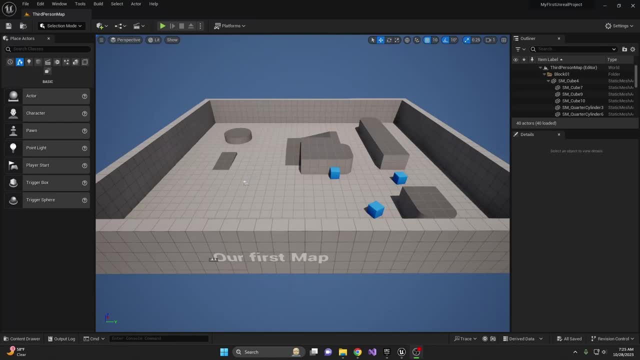 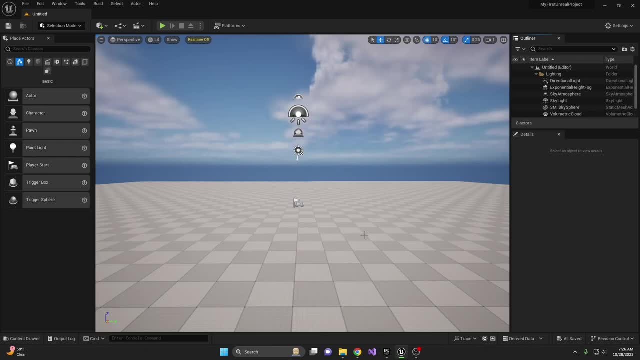 basic. Create Basic will create a new level with a floor, some lighting and a few other extras that make the scene feel more alive, And save your level under file: save current level. Go ahead and, in the content folder that is already selected, right click into this area. make a new folder. 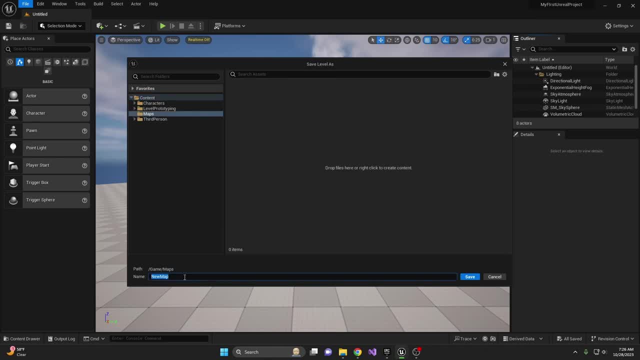 and call it maps. Select your new maps folder, rename your map and hit save Our first map. Now keep in mind, Unreal Engine doesn't like space bars in these kind of things. So if you want to separate words, I would just do that. So if you want to separate words, I would. 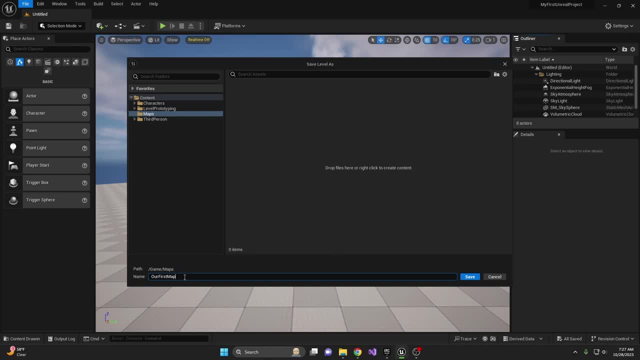 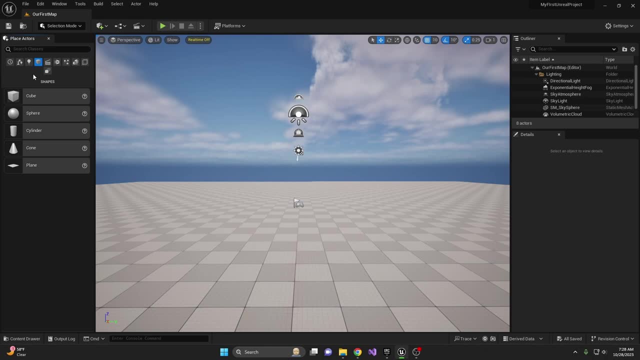 suggest using an underscore, Or just ignore the space and capitalize each new word. Now, on the left panel, go to shapes. This is your basic building block store. You have various shapes, including a cube, sphere, cylinder, cone and a plane. These shapes are more than enough. 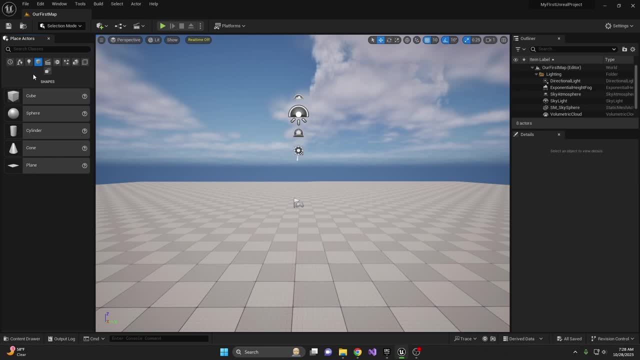 for you to prototype a level before you have any art assets done. So let's play around with them. First take a cube, drag it into your scene, Go ahead and use the blue arrow to move it up until it's flush with the floor. Then let's take a sphere, drag it in as well, And 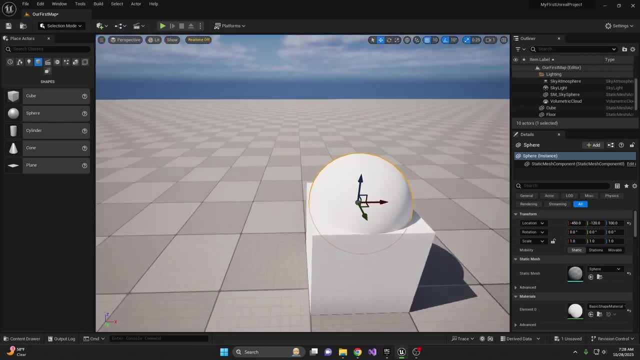 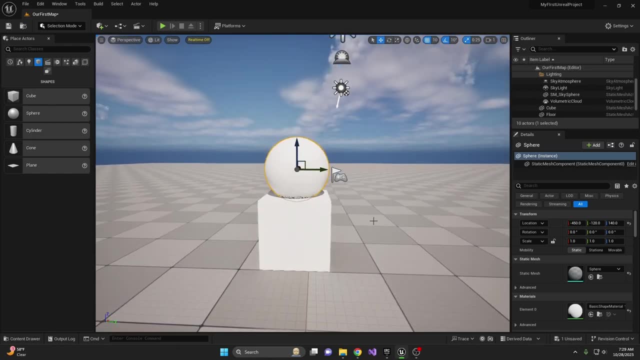 place it on top of the cube. If you need to, you can move in closer. Make sure it's nice and centered above the cube, Move the sphere up a little bit as well, And now you made yourself a little pillar, or statue, or whatever you would like to call this. Do you remember the scene? 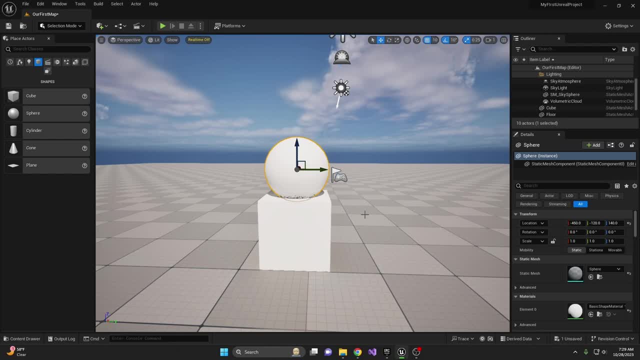 hierarchy we talked about in one of our previous videos. Go ahead and make the sphere a child of the cube. This allows us to always move it around together From here. you can then manipulate this geometry in multiple different ways. using the W, Q, E and R key, You can change how. 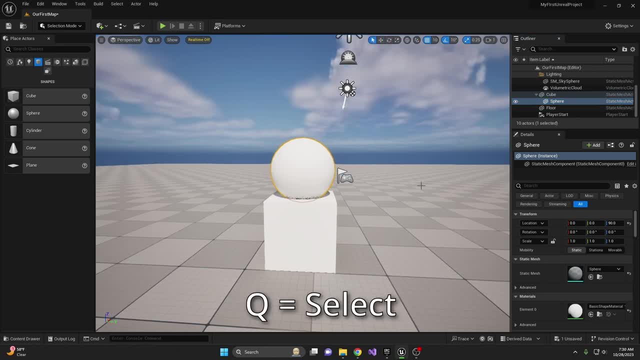 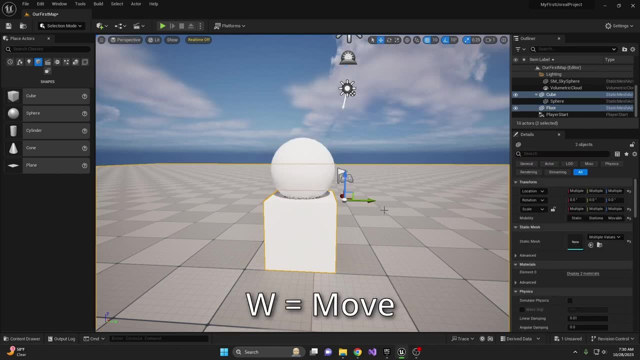 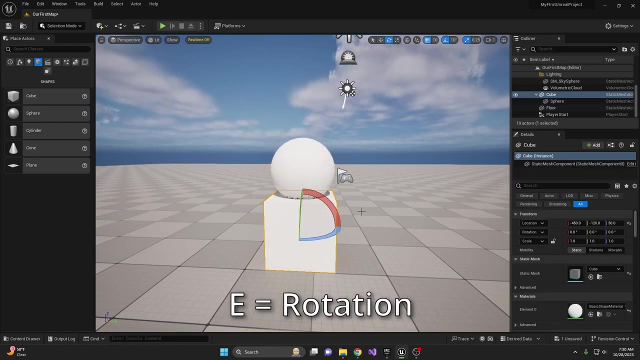 you manipulate an object in your scene. With Q, you enter selection mode. This allows you to select objects. You hold control while clicking on an object, you will be able to select multiple objects. W is the move tool. Using the arrows, you can move the objects around. E is the rotation. 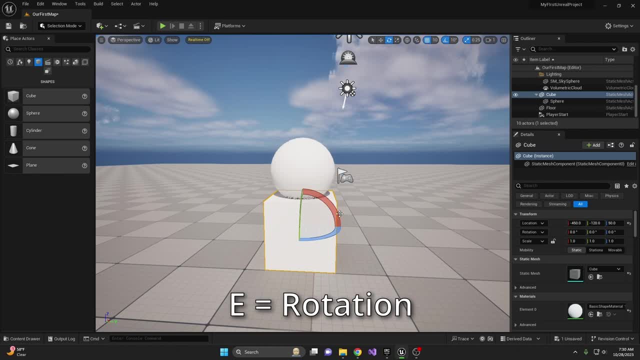 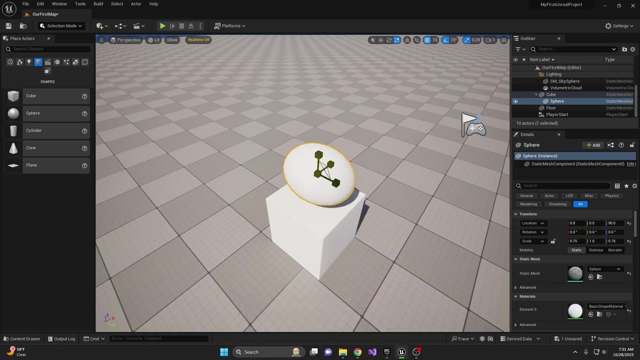 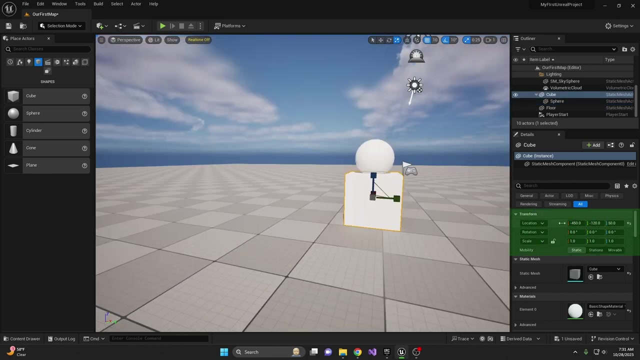 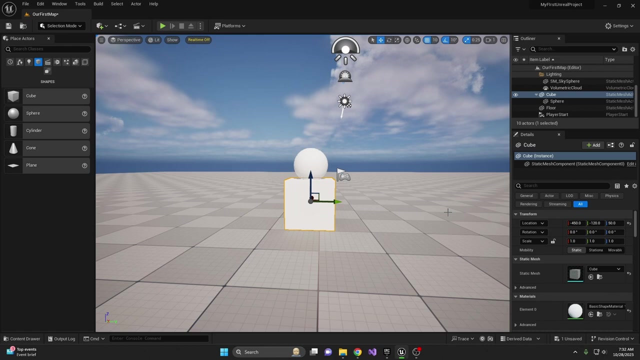 tool. This allows you to rotate your objects into your desired angles, And R is your scaling tool. You can change the scale of your objects, Or you can also go into your details panel of the selected object and manipulate the location, rotation and scale. With this alone you could create a decent block out of your level. But let's. 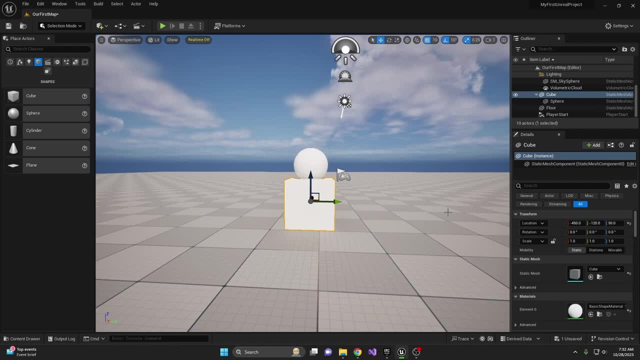 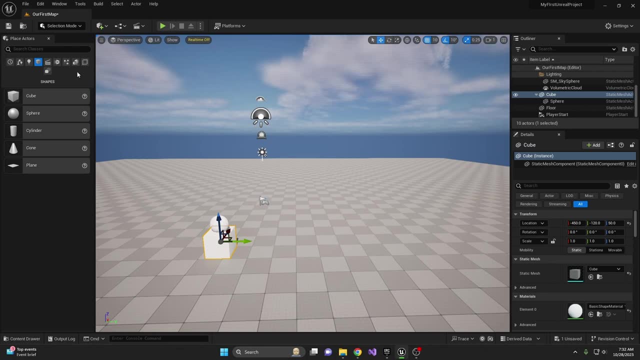 take it a step further and take a look at BSP brushes. They will allow us to create much more detailed objects that could give our levels a much better feeling. Go back to your place actors panel on the left side and this time choose geometry. Here we have similar shapes as 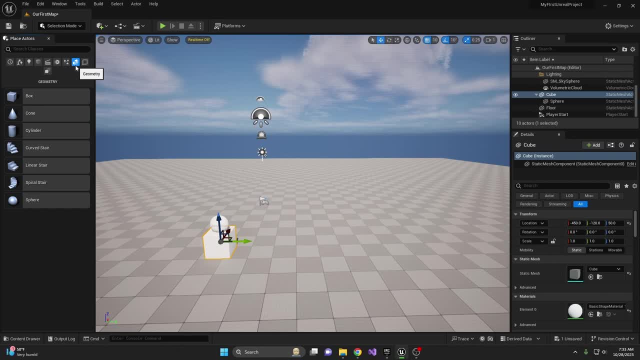 the shapes tab with addition of different types of stairs. But for now let's create a room for our level. Drag a box into the viewport. Do you notice the difference between the two cubes? we've already added In our details panel. you will now see all the details for the box we just added. 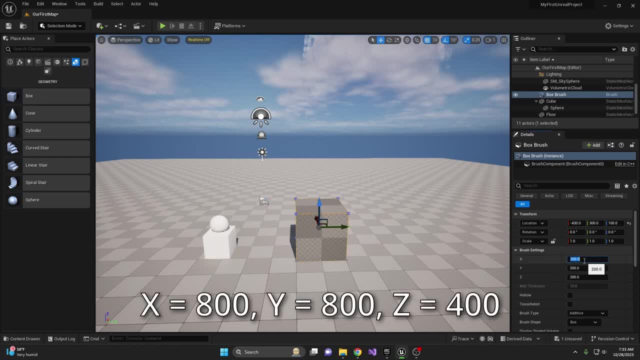 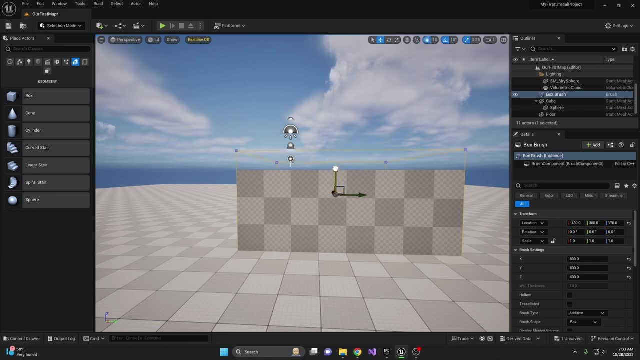 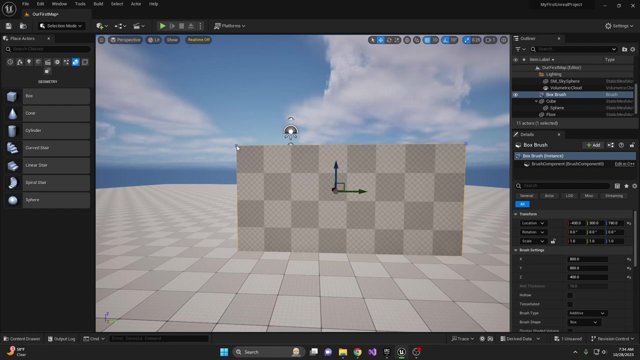 Under brush settings. we will go ahead and increase the X, Y and Z to 800,, 800, and 400.. Then go ahead and move the box up so it is flush with the floor, maybe down just a little bit. You can see the small blue squares around your box, which would 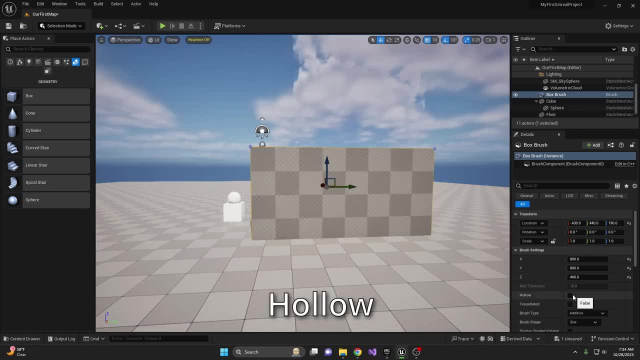 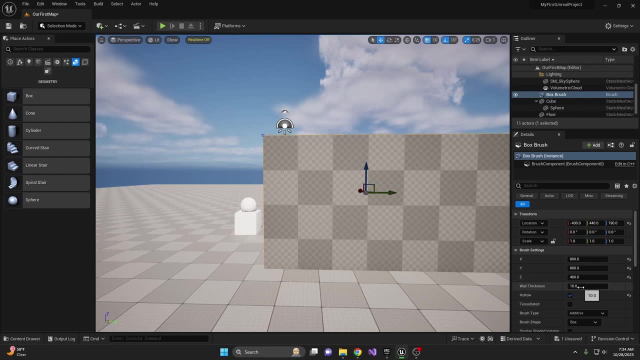 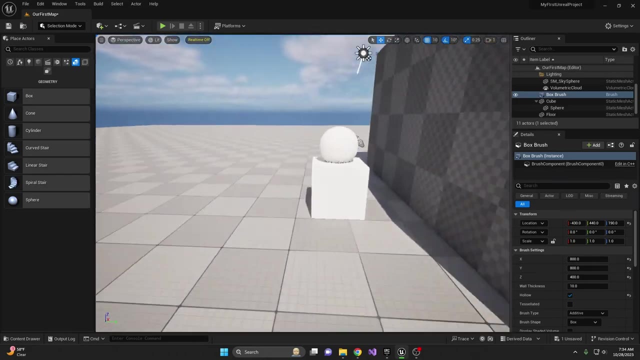 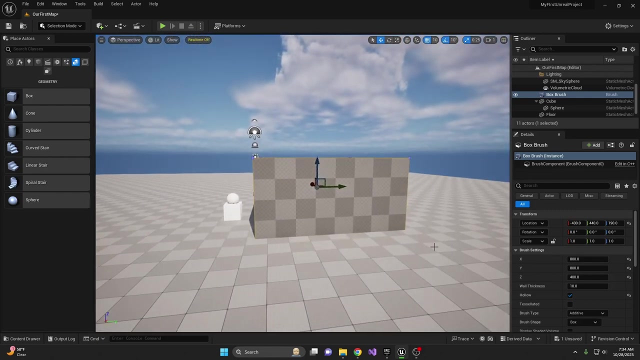 make it much easier to align inside of your world. Next, under brush settings, check the hollow button. This will hollow out the cube and create a room for us. You can then change the wall thickness to your desired thickness, But without a door we can't get into our newly created room. So let's add another box into our 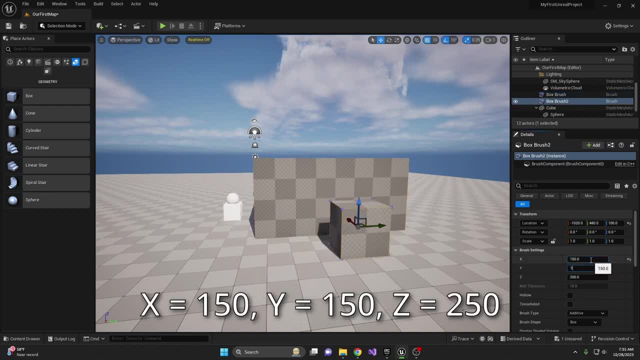 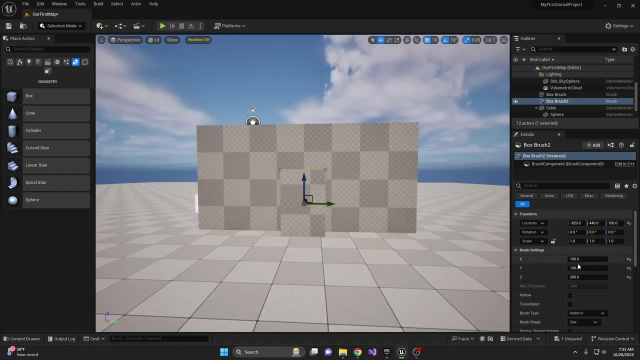 scene. Change X, Y and Z to 150,, 150, and 250.. And drag the box into the wall so it overlaps where you want to place the door. Next in the details panel, move down the brush type and change from. 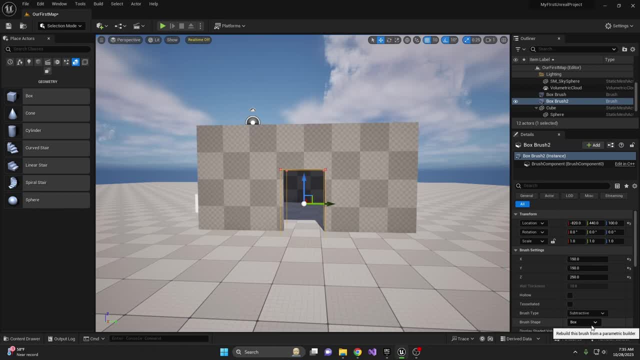 additive to additive And then in the details panel, move down the brush type and change from additive to subtractive. This will then cut out an exact section of the box you are using. Congratulations, you just built your first room. Now you will notice in the world outliner. 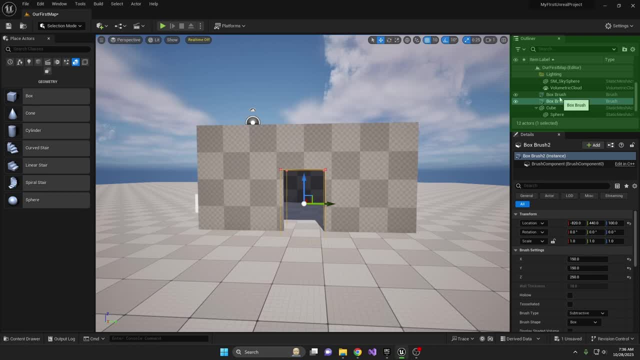 there is a small plus and minus next to the box brushes that we used. That way you can see if it is an additive or subtractive object. Now go ahead and pause the video and add some windows and decorate the room a little with the pillar you just created One little. 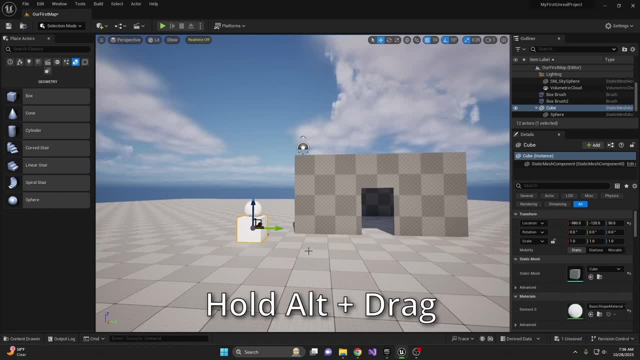 quick tip before you get started. You can duplicate objects in your scene by pressing Alt and dragging them around. This, however, will not take the child with it, So in order to take the child with it, you will have to select both objects. 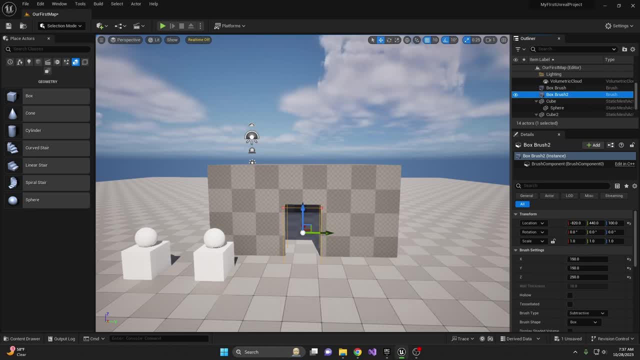 Alt and drag. Keep that in mind. for the windows you are about to create, You can just duplicate the box you already have set to subtractive, or bring in a new box. Or if you want to use a different shape window, go ahead and do that as well. Now a quick recap. BSP brushes serve as 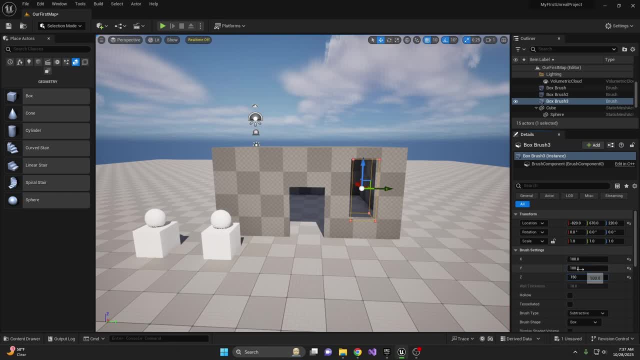 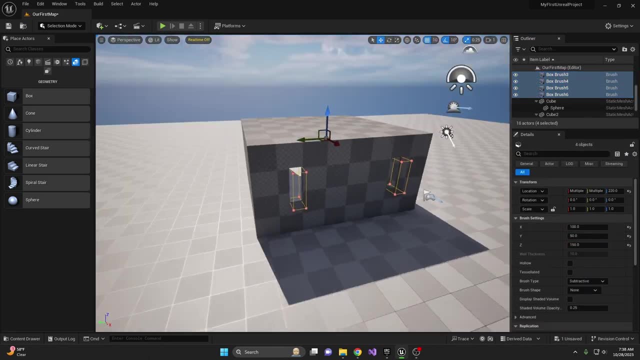 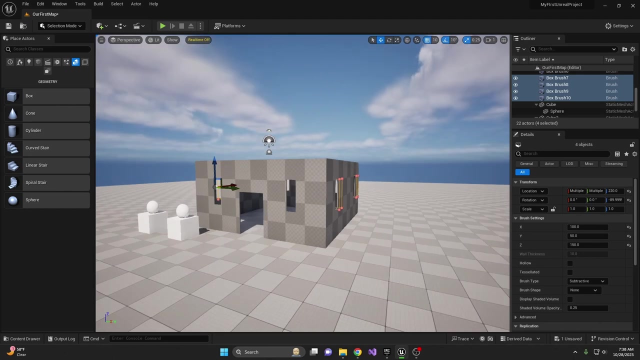 the basic building blocks of a level in Unreal Engine. They are primitive geometric shapes like cubes and cylinders that you can manipulate and use directly within the Unreal Engine editor. These brushes can be used for level prototyping and basic geometry construction. They are commonly used for grayboxing or rough layout planning to quickly prototype your level's. 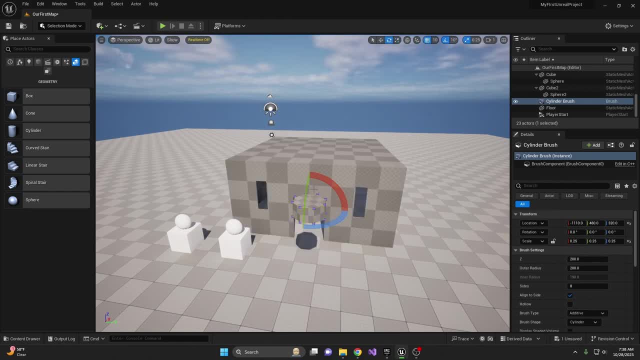 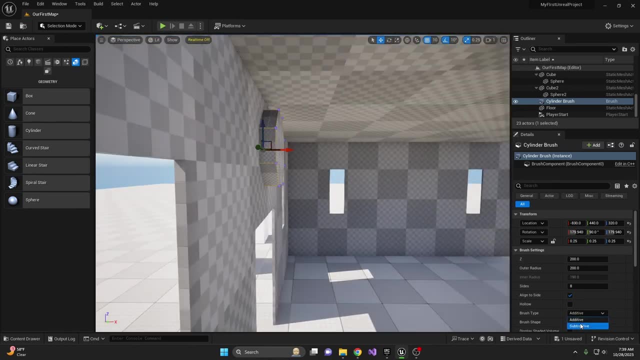 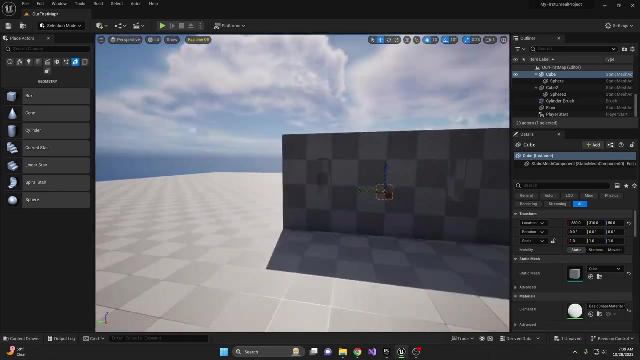 spatial arrangement. This allows you to visualize and iterate on your level's design before finalizing it with more detailed assets. While BSP brushes are useful for blocking out level geometry, Epic Games and any reputable game development studio would recommend to eventually replace them with static meshes for detailed and optimized environments. 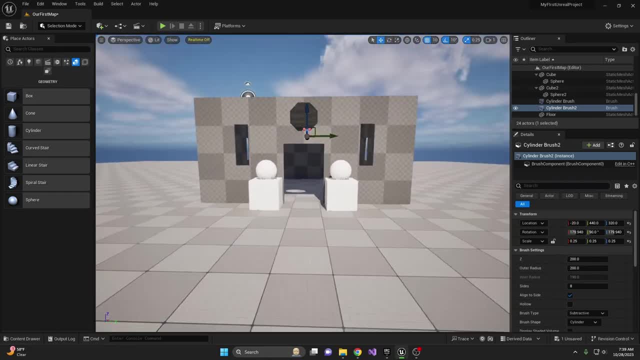 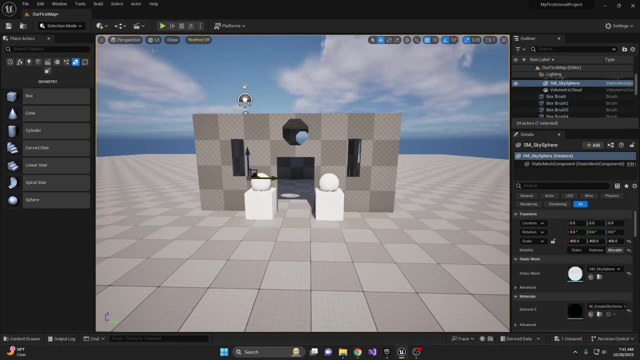 BSP brushes may not be suitable for the final polished version of a level, unless, of course, you are planning a level that is supposed to look like this. Once you are done, don't forget to save your level once again by hitting the save icon to the top. 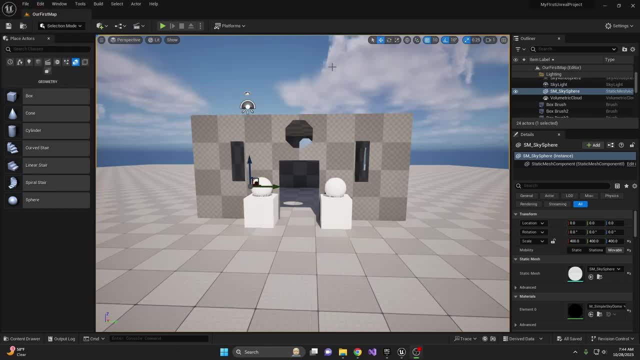 left or going under file and save current level. Once you finish building out your little room, go ahead and hit the green play button up here. This will allow you to play your level in the viewport editor, or right click into your scene and click play from here.